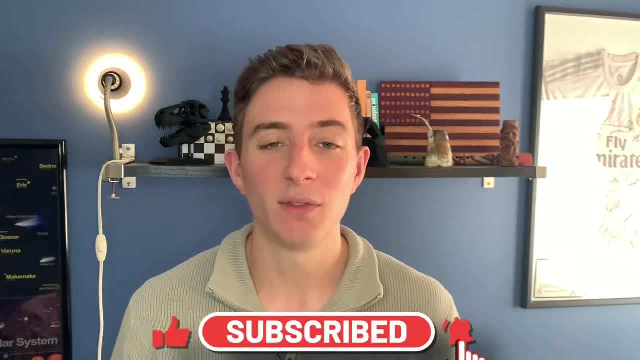 If you want to stay up to date with the current market here, then subscribe below and tap that bell for notifications so you can be the first to know about the current market here. current market in northern virginia. my name is tim and you know the team and i here. we get calls. 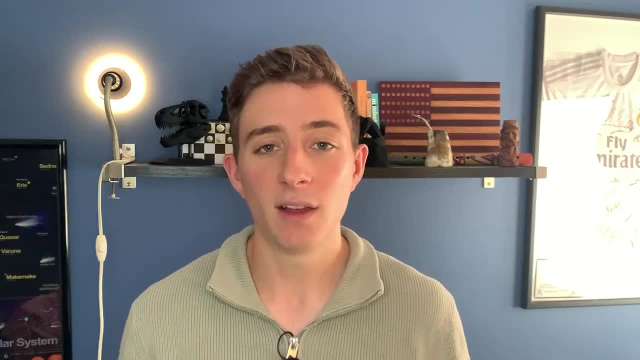 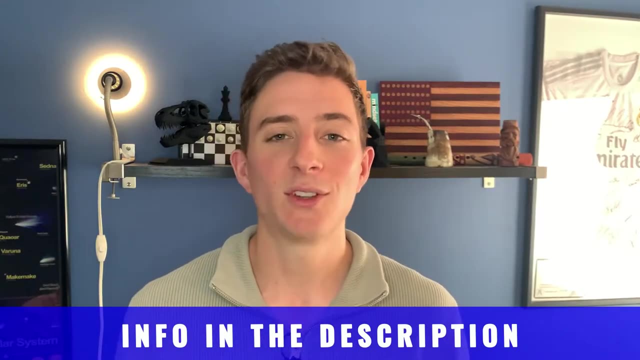 texts and emails from people just like you, looking to make their move, and we love it. so, whether you're moving in a day, a year or any time in between, give us a call, shoot us a text, send us an email, schedule a zoom call, even whatever is most convenient for you. guys happy to help you. 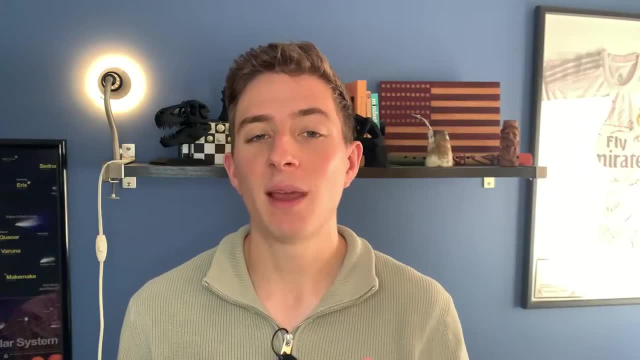 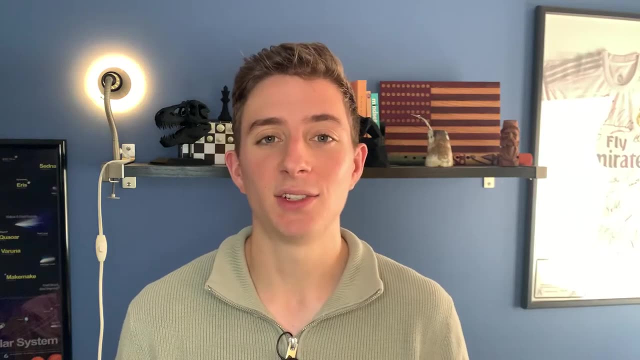 make that smooth move here to northern virginia, getting started straight off the bat. looking at california versus virginia now i am going to be a little bit biased towards my area. i've been living here for the last 17 years, so it's been doing something. right for me, right, but i will. 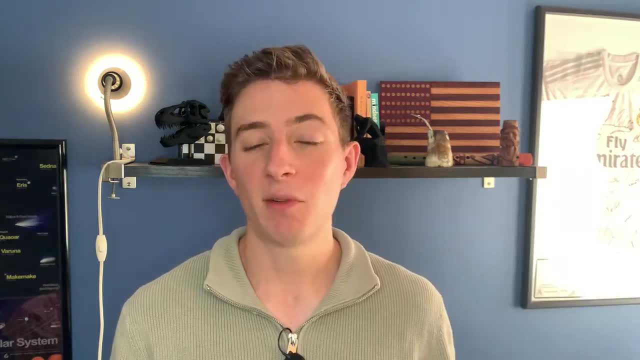 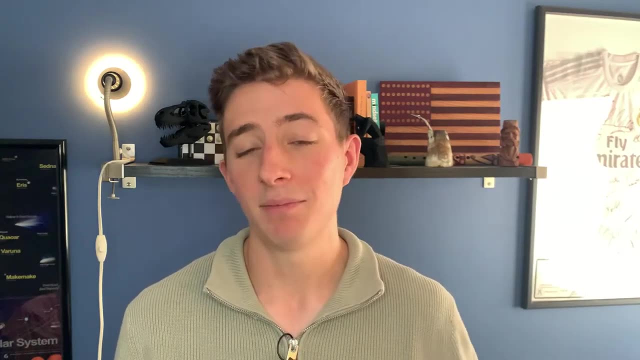 buy down to california. i will give credit where it is due. it is one of my favorite places to go for vacation, visiting friends, family. i mean, the weather is great, the nightlife and the things to do out there are just top notch. not many areas can really compete with it, but you know, if we roll back the clock 10, 20 years. it was probably one of the best places to live on earth. hence why around 40 million people didn't migrate over there and you were even able to retain them. but now, over the last five to ten years, especially during the pandemic, we're seeing the trend completely do a 180. more people are. 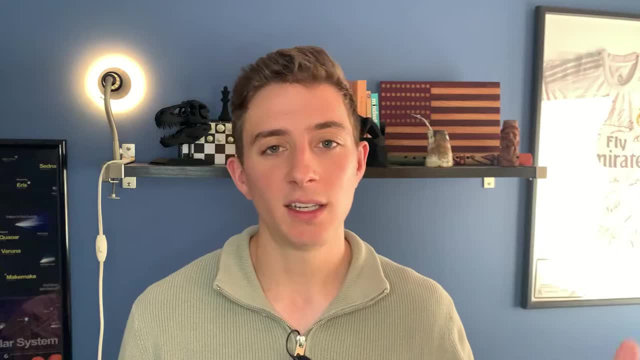 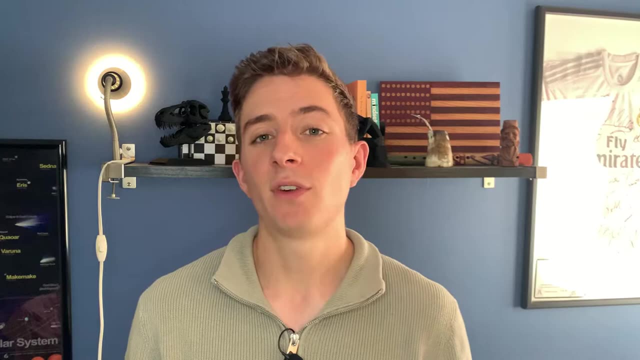 moving out than actually moving in. the growth rate is continuously on a downward trend. how long is that trend going to last? we don't really know, but that's kind of what we're seeing right now. now we always try to leave room for objectivity and facts and, factually speaking, california does. 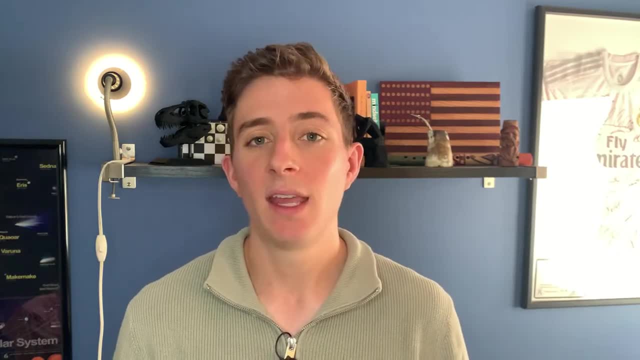 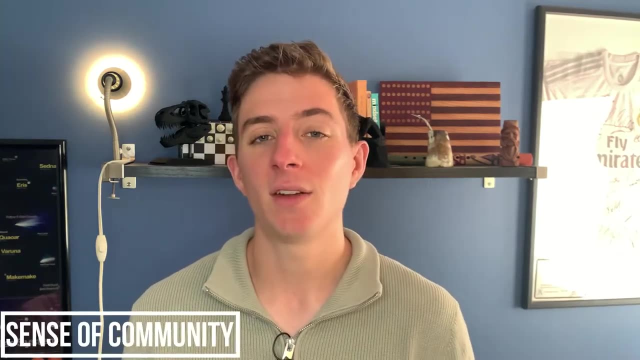 have things going for it that not a lot of areas can really compete with, but also northern virginia does have things up its sleeve that california can't really compete with either, one of them being the sense of community that you get out here in virginia, which is probably one of my favorite things. 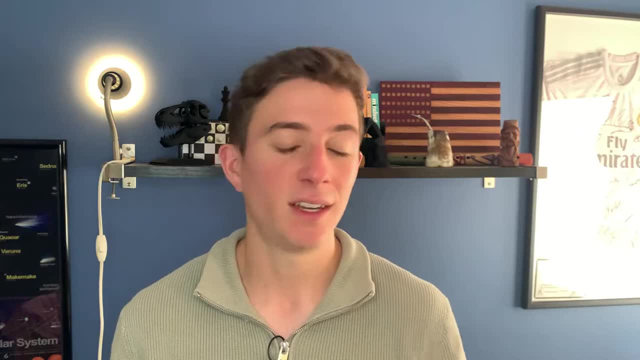 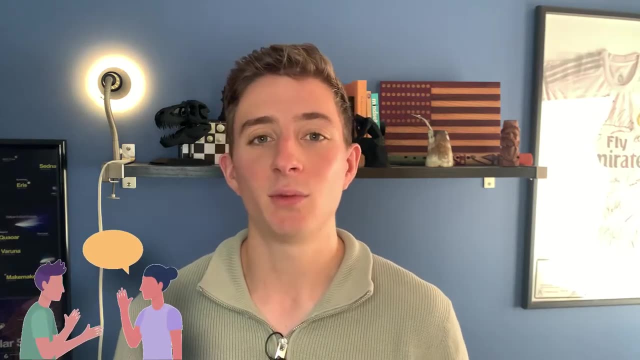 even though northern virginia is a little bit more of a city feel it is a metropolitan area. at the end of the day you could still be strolling down your neighborhood or your city and more often than not you'll spark up a conversation with a neighbor or a stranger that you've never even met or at 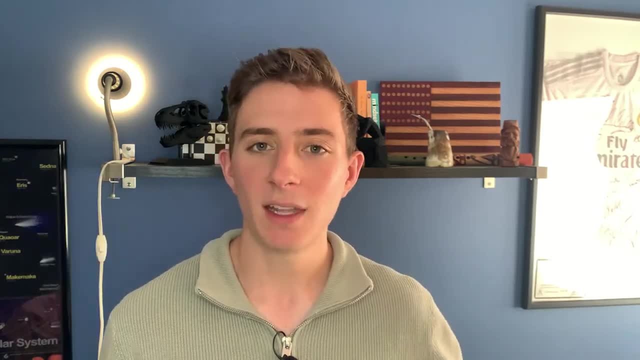 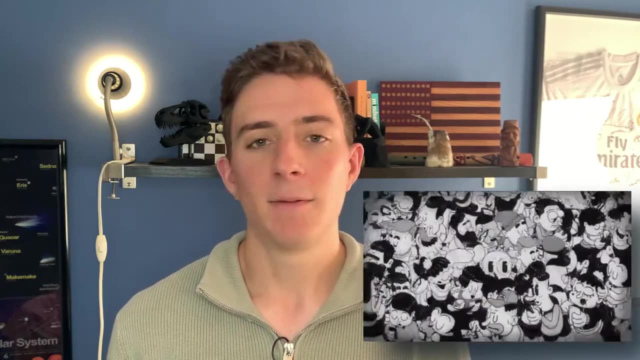 least get a wave and a smile from somebody where, in more populated areas in california like los angeles or san francisco, you know, when there's so many people bunched up in one space, from my experience even it's not hard to get a wave and a smile from somebody, but it's not hard to get a. 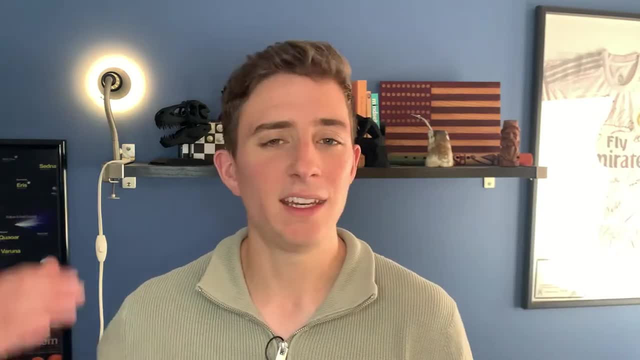 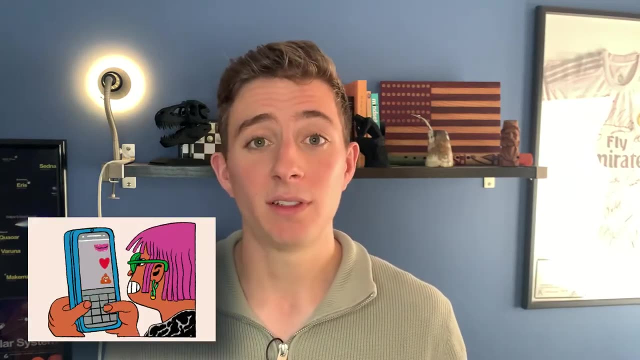 wave. not just los angeles, of course. even if you go to new york city or any capital of any other country, people are a lot more on edge, kind of in their own clique, a lot more tunnel vision, not really receptive to everything that's going on around them, and i think a lot of that does. have to do with the fact that you know your senses are definitely heightened when you're in these areas, right especially when the homelessness rate is the highest in the country in california and the crime rate tends to stay above the us national average, whereas here in the whole state of virginia. the homelessness rate tends to stay at around one percent and the crime rate tends to stay below the us national average. so comparatively, looking at both states from kind of a bird's eye view, yeah, virginia is a lot safer in comparison to california, but you also need to take that with a grain of 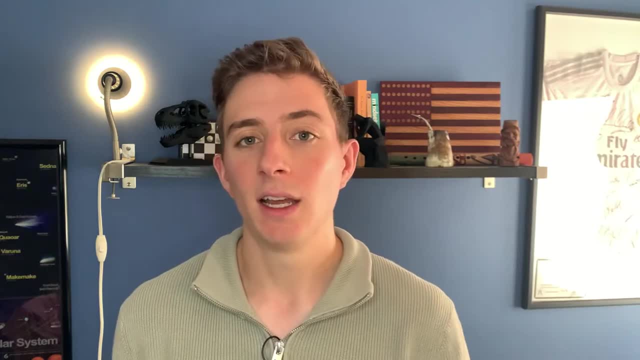 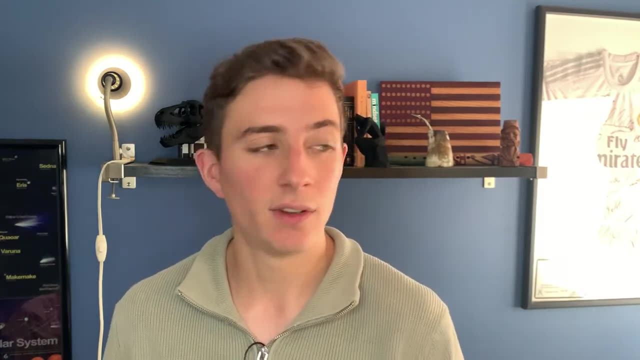 salt. there's a lot less people here, the state is a lot smaller, but also it also depends in what areas you're looking at, right, because there's going to be pockets in virginia which aren't very safe and there's going to be pockets in california. they're going to be very safe, for you. so it always depends on where you're looking. now, if we look at the public school systems that you get in each state, the state of virginia and northern virginia provide you with some of the best public schools that money can actually buy, especially in fairfax county and loudoun county. 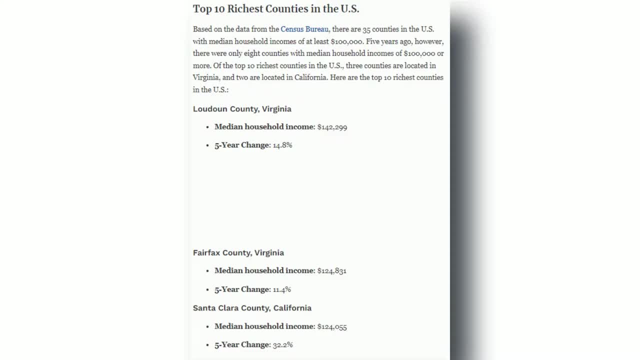 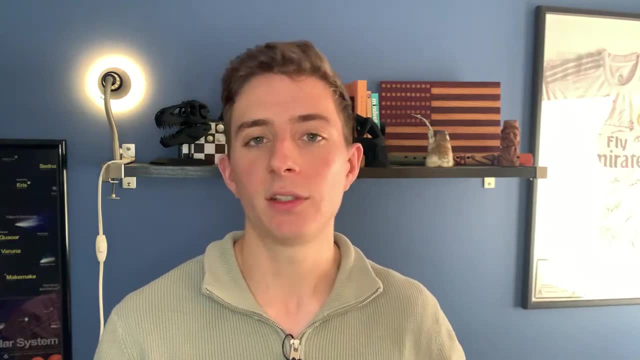 which are considered to be some of the most affluent areas in the country. they're going to give you some of the best public schools in the country right, whereas in california, if you go to the really affluent areas, you're still going to get world-class education out there. but the disparity tends to be a lot more significant from the more affluent areas to the less affluent areas, to the less affluent areas, to the more affluent areas to the less affluent areas, whereas in virginia, the more affluent areas and the less affluent areas, that disparity isn't as significant. you know, they kind of bring each other up and even throughout the whole state. 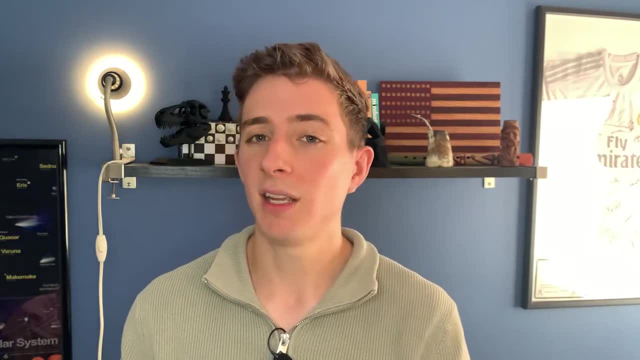 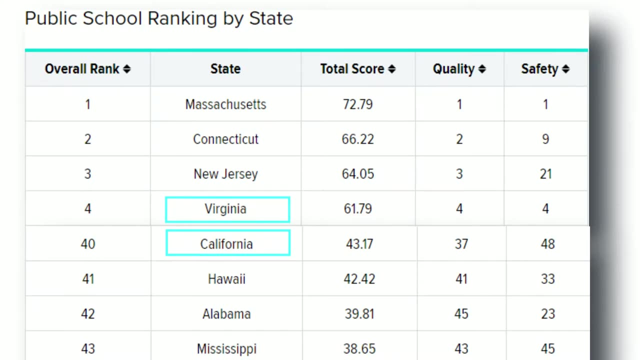 of virginia, that's going to be the case, hence why the whole state is typically ranked in the top five with the best public school systems in the country, whereas california is typically ranked in the top 40 out of the 51 states, and those stats are determined by things like funding. 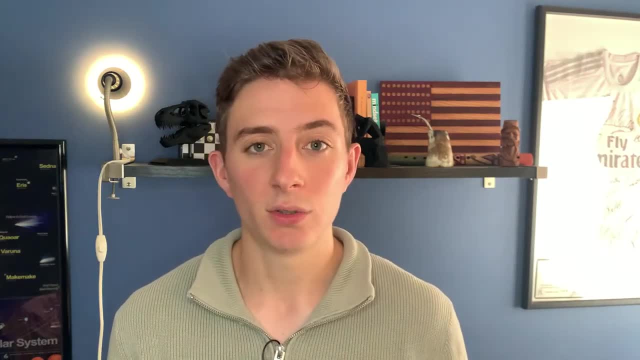 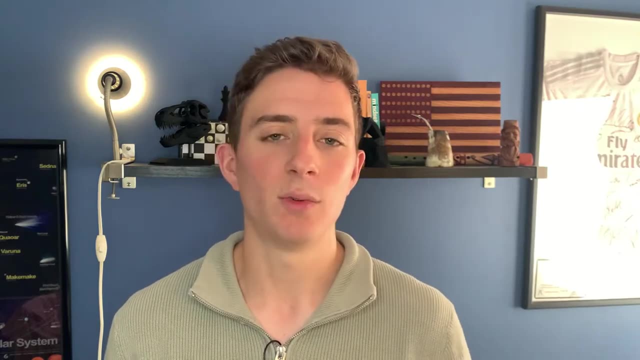 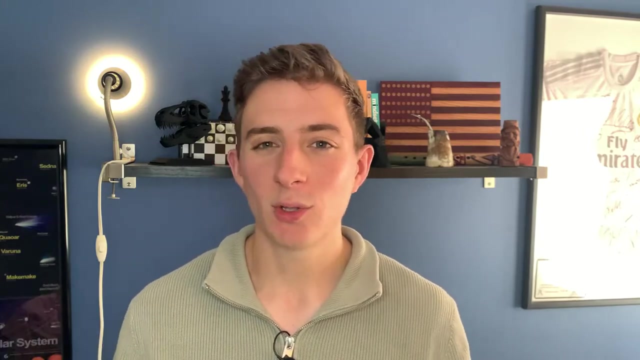 performance, class sizes and instructor credentials. so so, more often than not, you're going to find much better school systems in virginia rather than california. but, as i mentioned, it always depends on where you're looking. now, looking at the cost of living of both areas, now you get benefits in both states. it really depends on what it is that 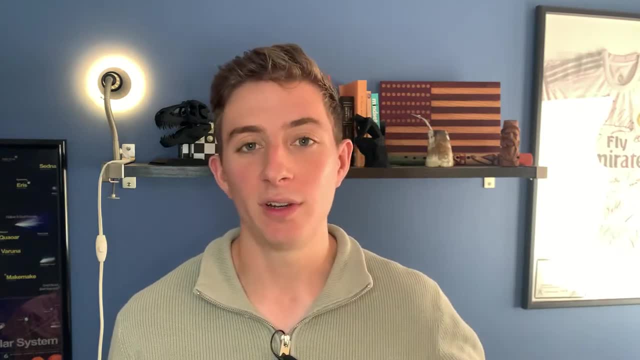 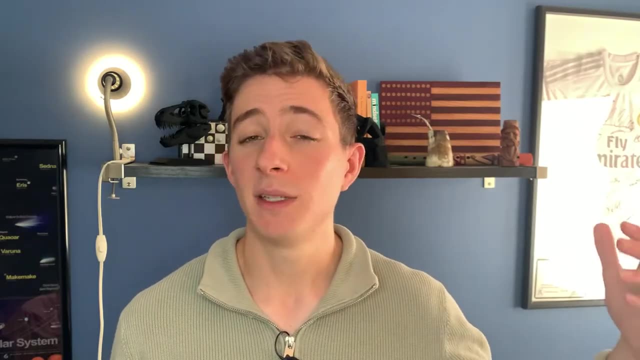 you value. i know a lot of young professionals. they love california, especially if they're just out of college- all the nightlife, the great weather and stuff like that. as time goes on over the years, the demand in california has been so high that it's been driving up the cost of living not only in real estate but in everything. 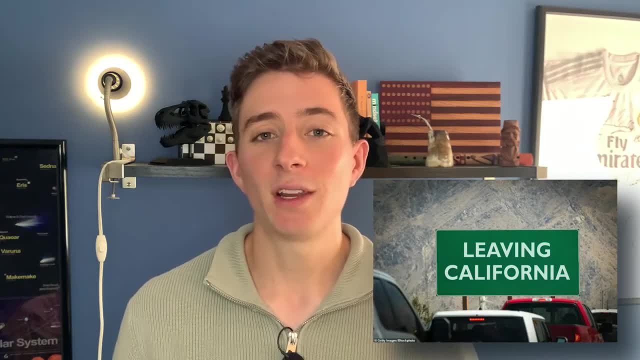 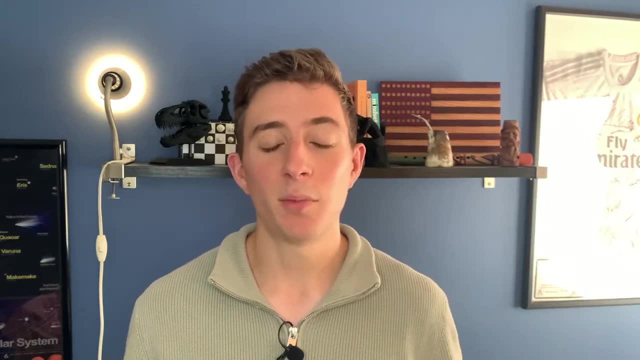 and uh, you know it's been pushing a lot of people out of the market, especially for regular families. it's become less and less sustainable living a healthy and prosperous life out in california, so many of them are pushing out to different states and, as i mentioned, more often than not northern virginia does end up popping up on their radar, even though northern virginia is still considered to be one of the most expensive places to live in the country. comparatively to california, it's still rather affordable now if we look at some of the more basic sort of things you're going to be. spending your money on. you're going to be spending a lot of money on your home. you're going to be paying around nine percent more on restaurants in california, around ten and a half percent more on groceries, five and a half percent more on transportation and around nine percent more. 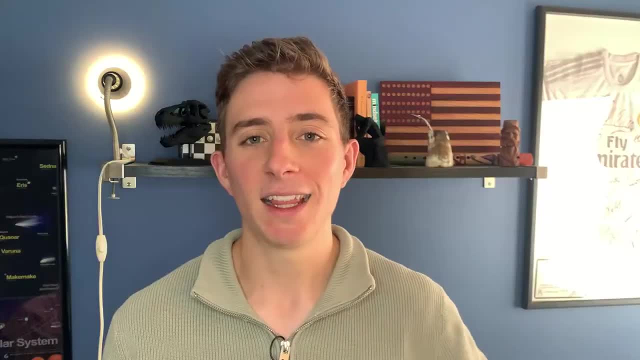 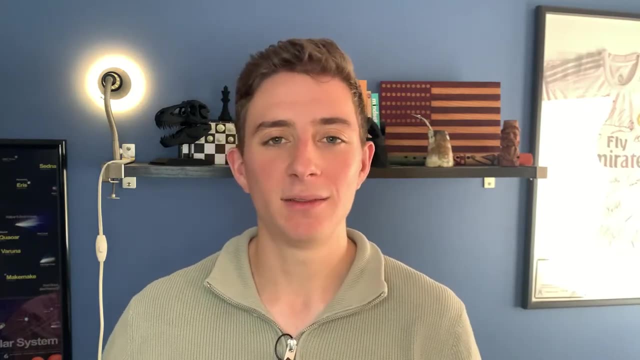 on sports and entertainment, even though that's probably going to be the only thing that's really worth your money. out in california, you guys have probably the best sports uh teams out there, whereas in comparison to here, the sports scene is pretty abysmal. if you like the wizards, if you like dc united, you're going to be disappointed. 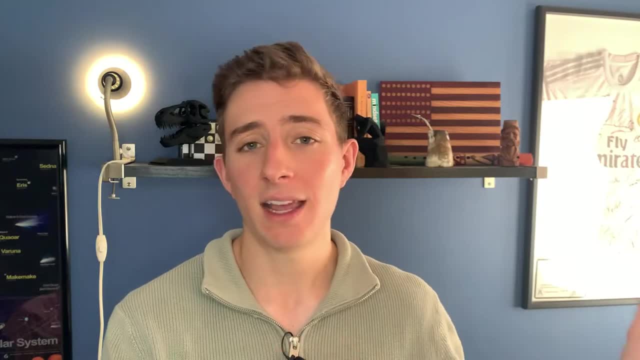 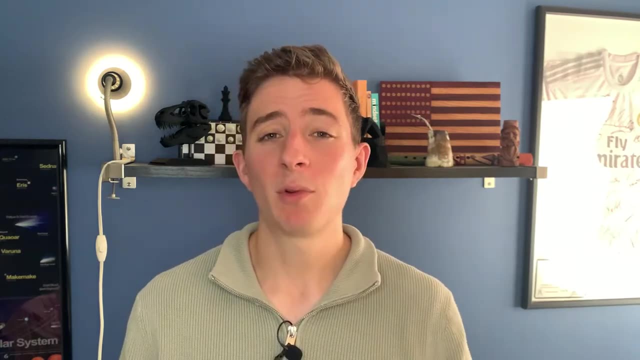 every single year pretty much. but if you really value that and you know california might be a fit for you- but is it really worth paying more in every other bracket? i mean that's up to you, but probably where you're going to be spending the most amount of money is going to be housing. 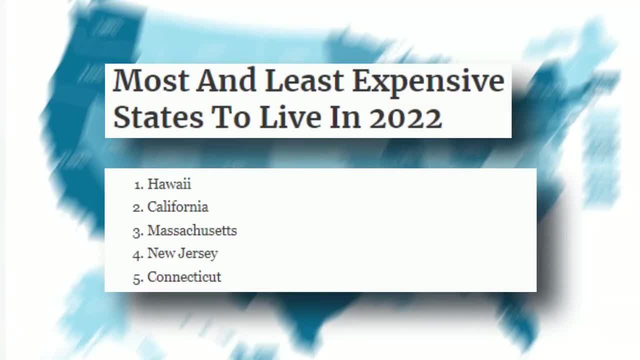 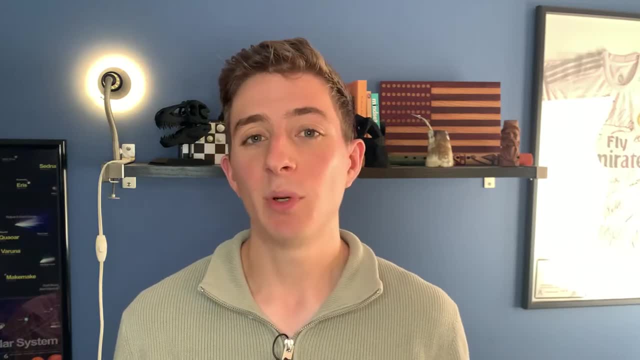 of course, california is considered to be the second most expensive place to live, right behind hawaii, and of course, as i mentioned, a lot of that does have to do with the demand and it's been pushing a lot of people out of the market but also driving up real estate prices. i mean the 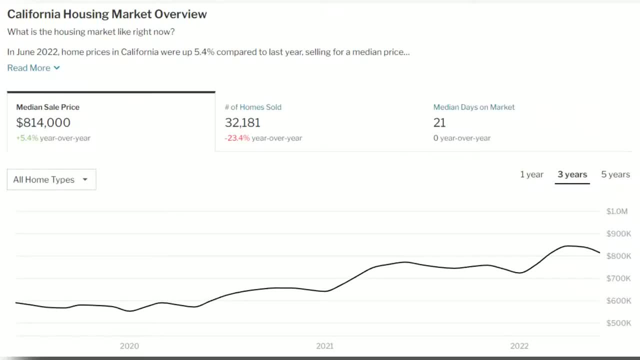 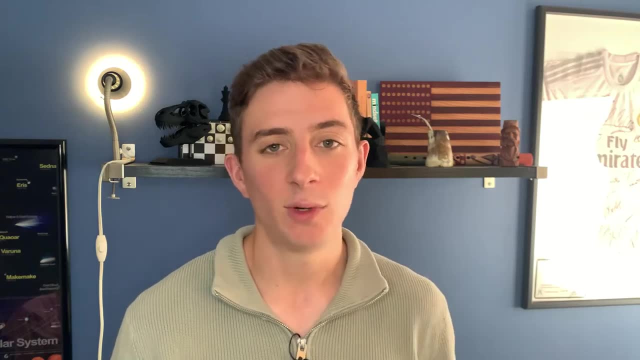 median home sale price in california is around 813 000. that's throughout the whole state. that's taken to account some of the most affluent areas, but also the more rural, less affluent area. so that's pretty significant, even though, as i mentioned, in northern virginia it's still one of the most. 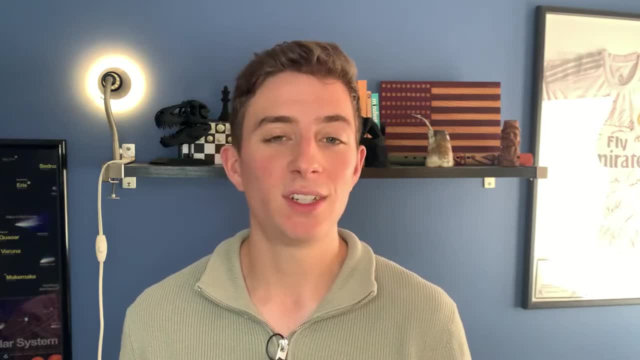 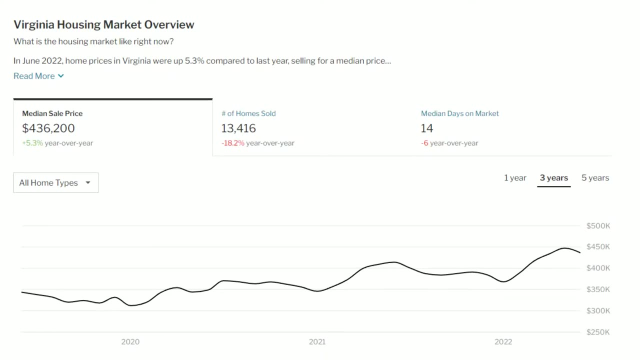 expensive places to live. the median home sale price all throughout northern virginia is around 600 000, whereas if you look at the whole state of virginia it's around 436 000, which is right around the median home sale price all throughout the country, and that has had a significant impact on 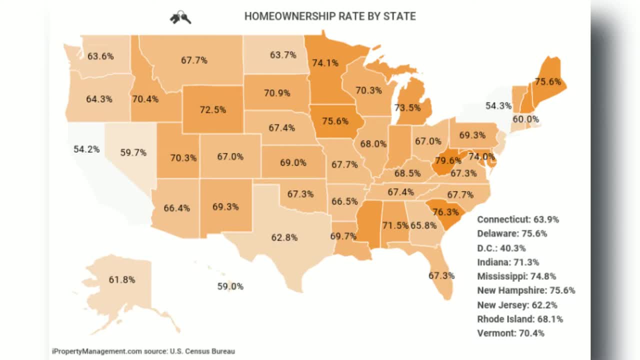 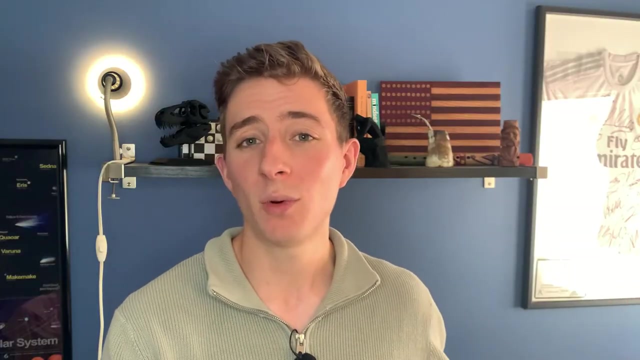 a lot of people, especially on the home ownership rate. i mean, if we look at the home ownership rate in virginia, it's around 65, 35, 65 own to 35 that do rent. vice versa, if we look at california, it's around 50- 50. and what that's kind of doing to a lot of people is the people that don't really want to move from california, they want to stay there, they want to live. but once they realize, oh shoot, i need to buy a house, two things end up happening: either they stay in california because they love it so much and they end up renting for the rest of their lives, or they'll be pushed out. 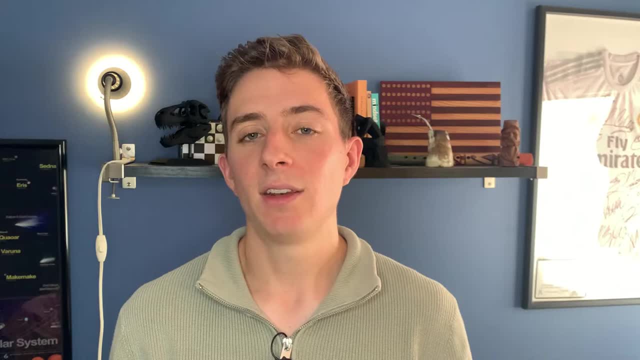 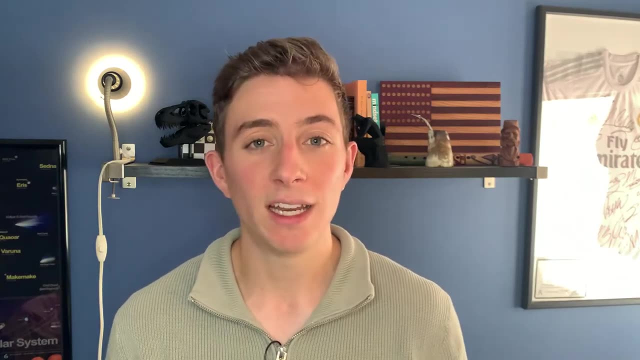 of the market and forced to find a home, uh, somewhere else and uh, you know that can be challenging for a lot of people doing and making a decision like that, and especially when the median household income is so low comparatively to the cost of living. i mean the median household. 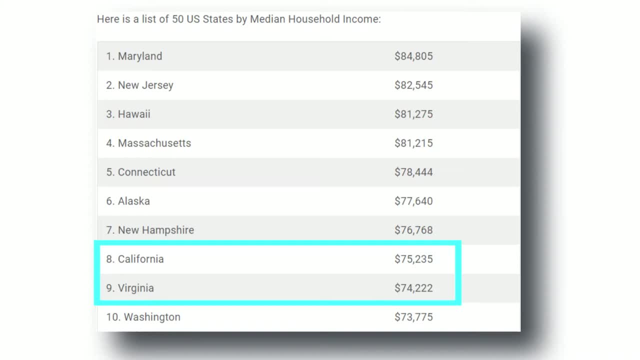 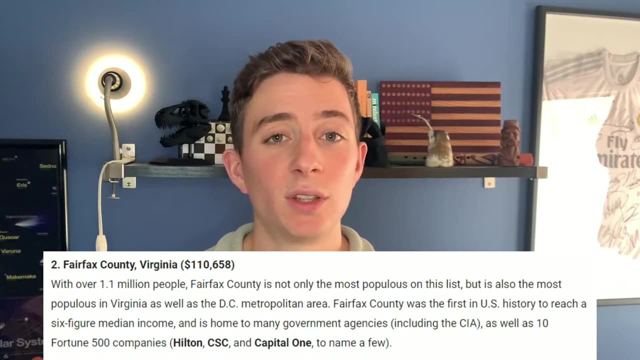 income from california to virginia is basically the same. it's around 75 000 for both states, whereas in a place like fairfax county we were actually the first county to reach a hundred thousand dollars in median household income in the country. so you're making a lot of money here. 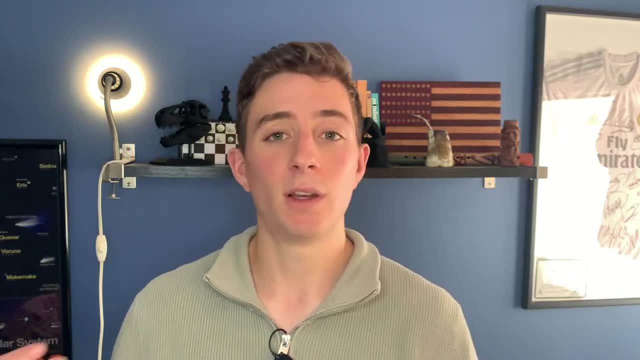 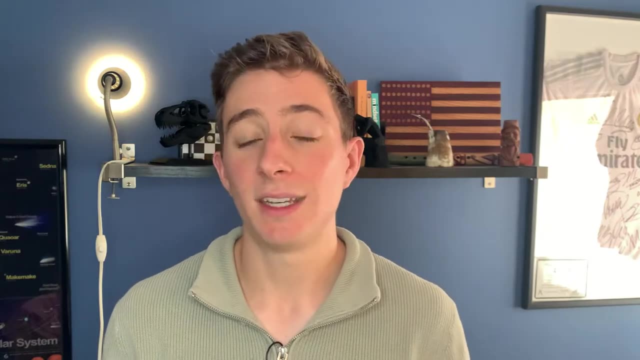 and you're getting a much bigger bank for your buck. hence why the the home ownership rate is uh, a lot higher in a lot of these uh suburban areas here, whereas california- the affordability just isn't there for many people. you're even going to be paying more on taxes in california in comparison. 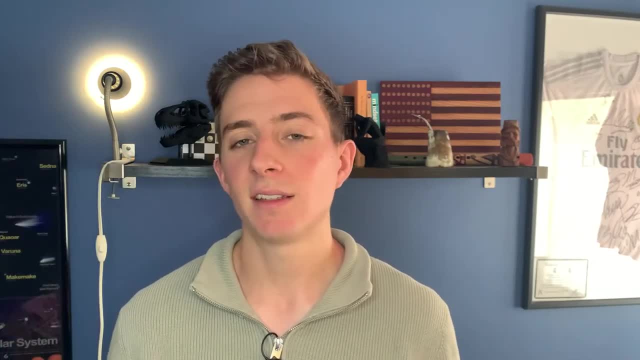 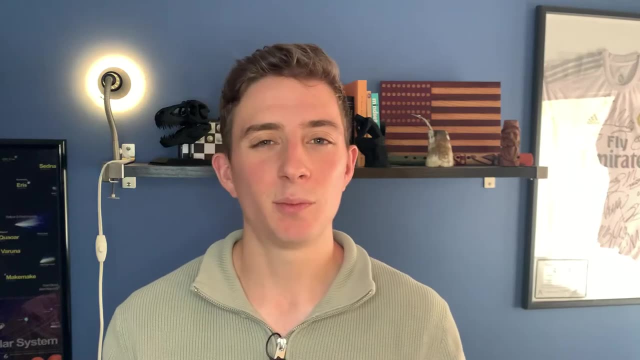 to virginia in pretty much every single bracket. you know sales tax isn't so significant if you're paying around one to four percent more in california, depending on where you live. same thing with property tax. it's pretty similar, but california tends to be a little bit higher. but 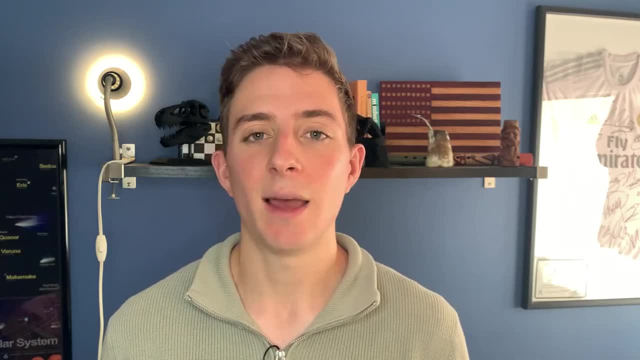 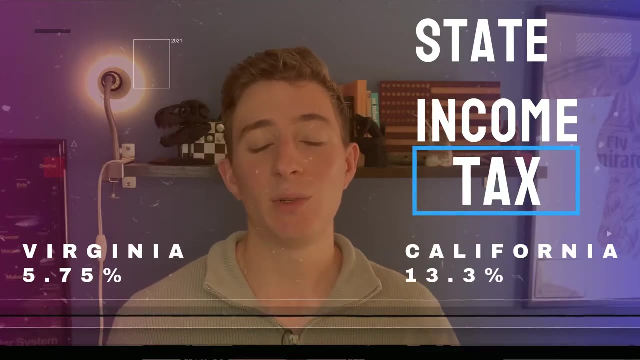 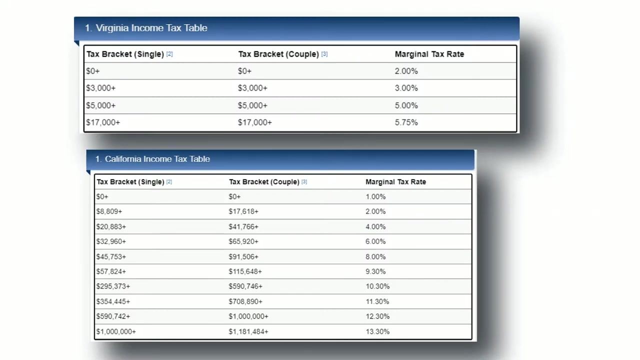 income tax is where the big disparity does tend to happen. you know, the highest marginal tax rate you get in virginia is 5.75, whereas the highest you can get in california is around 13.3. however, in virginia you reach that 5.75 benchmark once you make 17 000 for that tax year, and in california 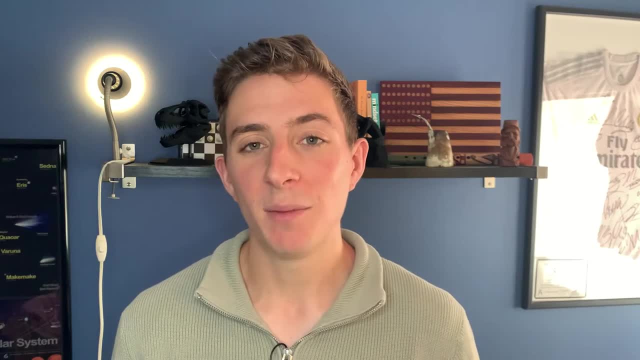 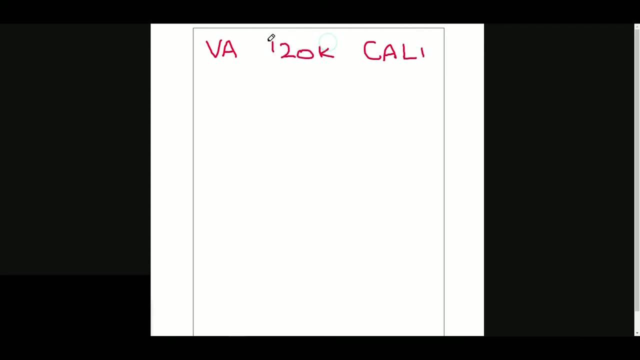 you reach that 13.3 once you make a million dollars. now most people aren't making a million dollars, so we're trying to get a kind of an example out there for you guys. that's a little bit more realistic. if we look at two people making the same amount in both states, we'll say around 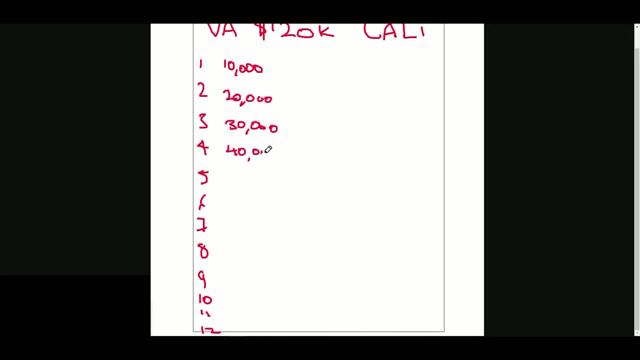 around ten thousand dollars a month. you know, in virginia if you make the first two months you're going to be paying around two percent. once you finally cross that 17 000 threshold you're gonna be paying 5.75 for around 11 months in california. is that for the first two months you're gonna be? 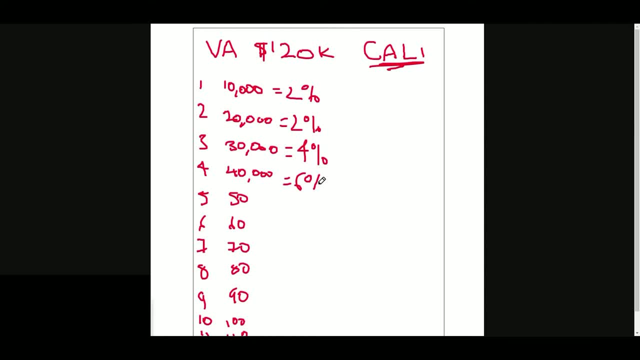 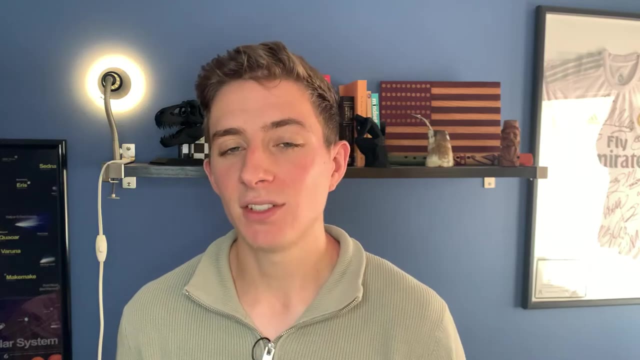 paying two percent on that ten thousand dollars a month. for the next two months you're gonna be paying four percent, then you're gonna jump up to six percent, eight percent and for the remaining six or seven months you're gonna be paying 9.3 percent on that $10,000 a month which, at the end of the tax year in Virginia, you're going to be. 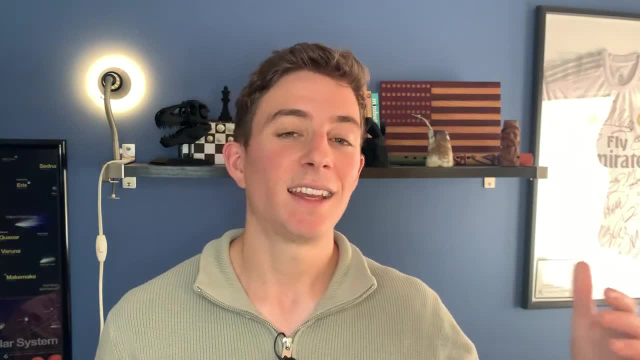 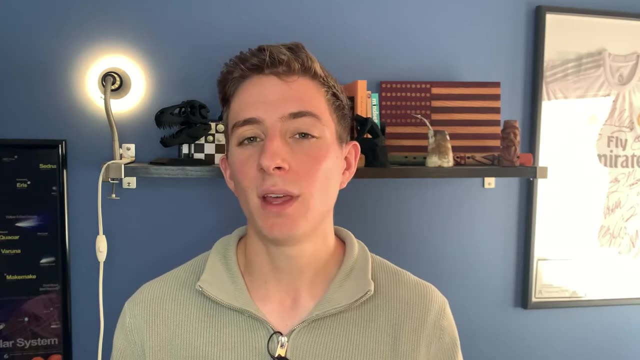 paying around $6,800 on taxes in California. You're going to be paying around $8,700.. Now that's around $2,000 at the end of that tax year And that's $2,000 that you could have been saving. 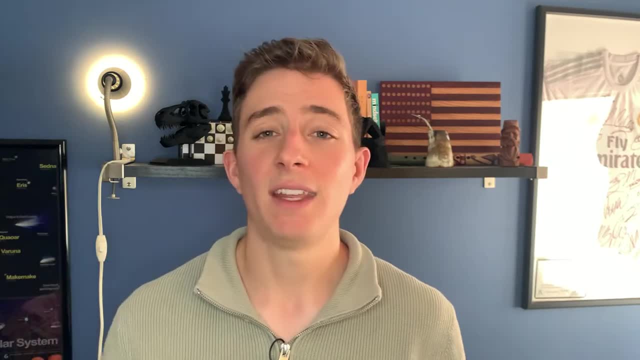 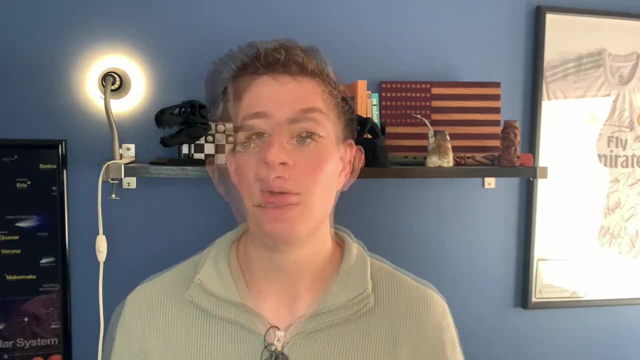 $2,000. You could have been investing, You could have been on vacation, You could have been spending that on anything else in a state where your money does tend to take you much further than a place like California. Now, big talk of the town, about California, big reason why people do love going. 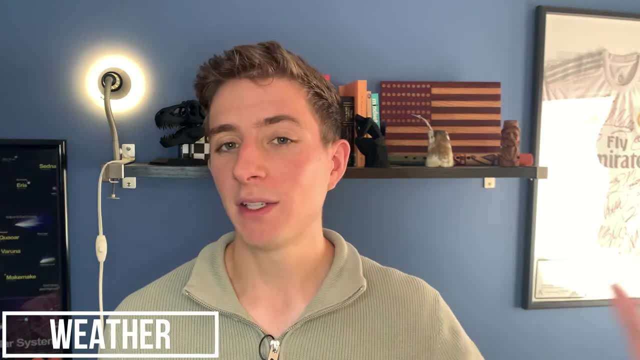 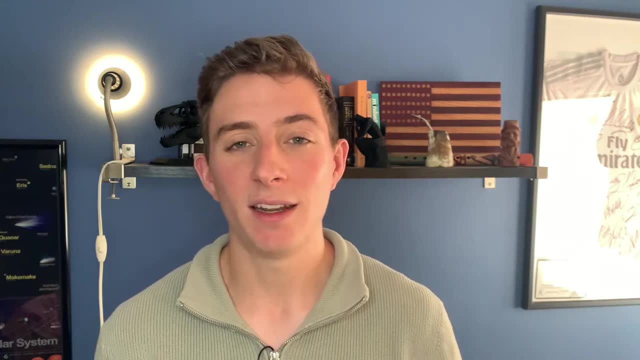 out there- And personally I love going out- there is going to be the weather. I mean especially in Southern California where the weather is a lot drier, you know you get 70 to 80 degrees day in and day out. You don't tend to get a lot of rain, Whereas in Northern California, I do know, in San Francisco and stuff like that. you get a lot more rain, It's a lot colder, So it's a little bit more balanced out, Whereas in Virginia I personally prefer the four distinct seasons that you get out here, And that's because you get a lot more variety to it. You get a lot more variety to it. 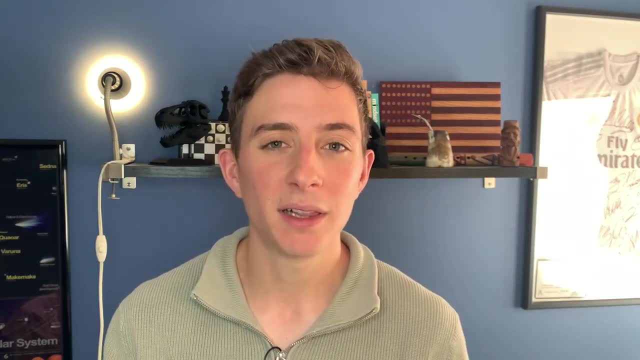 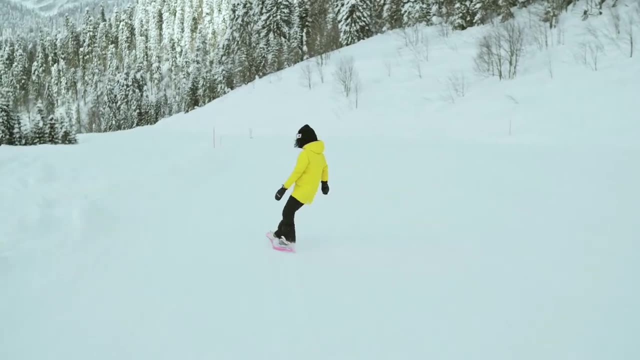 You know you can experience the same exact location in four completely different ways. You know you can go to the nearest mountain top when it's winter time and it's snowing, and you can take advantage of the ski slopes. You can go snowboarding, sledding, snowball fighting, whatever. 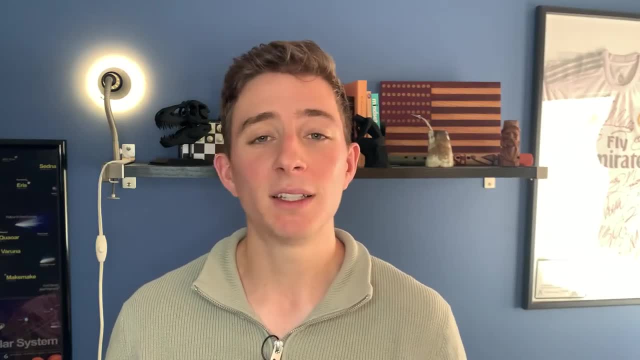 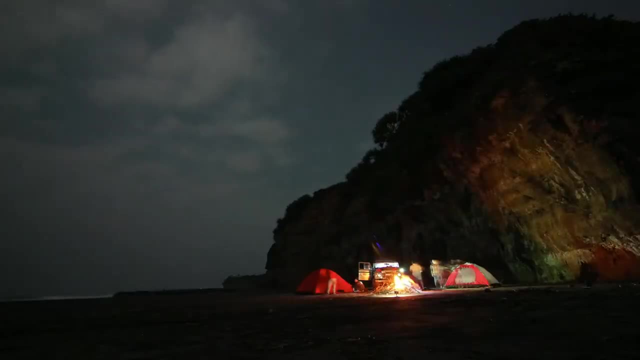 you like to do, You've got that at your disposal. Vice versa, a couple months later, you can go to that same mountain top during the spring, when the flowers are blooming, the trees are getting their color again and you can go hiking, mountain biking, camping, zip lining, whatever you'd like. 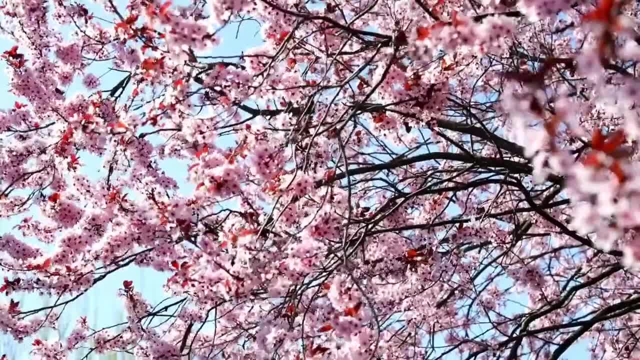 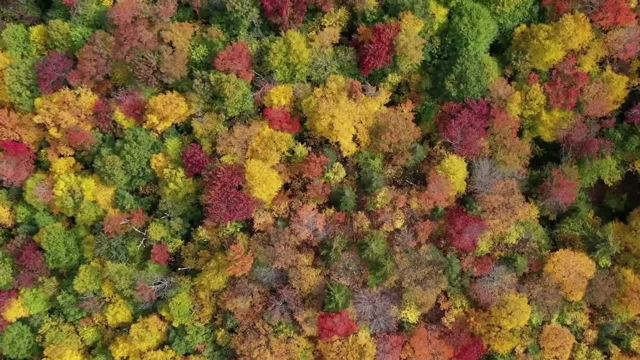 to do outdoors. That's going to be the best time to do it, And same thing with the snow. You can do that with the fall right, When the trees are changing colors and the weather's just perfect. the temperature is perfect. That's also going to be a great time to be going outside and doing. 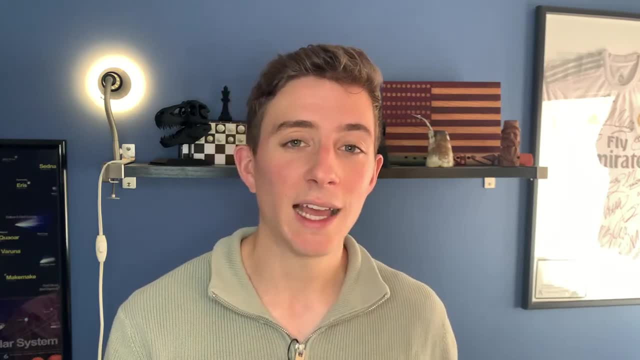 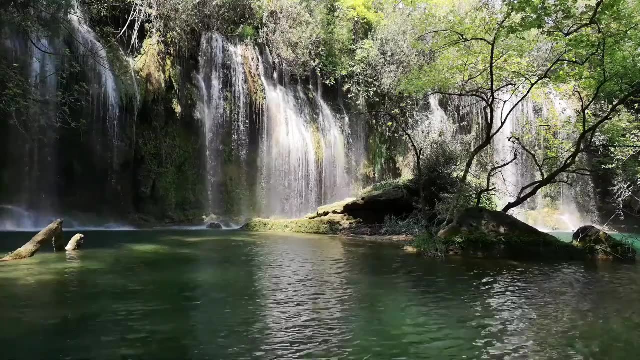 those outdoor activities, Whereas in the summertime, although it gets really hot and humid out here, we've got a lot of bodies of water, We've got the coast where you can go take advantage of the beaches, We've got waterfalls, rivers, lakes. I mean all of that you can take advantage of when 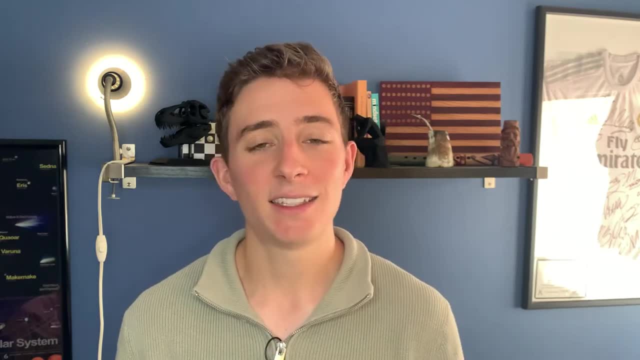 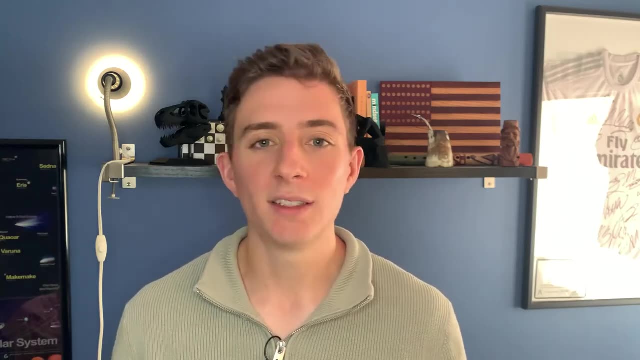 it's really hot and humid, Not to mention you've got a lot of neighborhood lakes that you can turn into ice skating rinks once it freezes over during the winter, So it's going to be a great time to. It just adds on to a much more nuanced sort of experience all throughout the year, which you 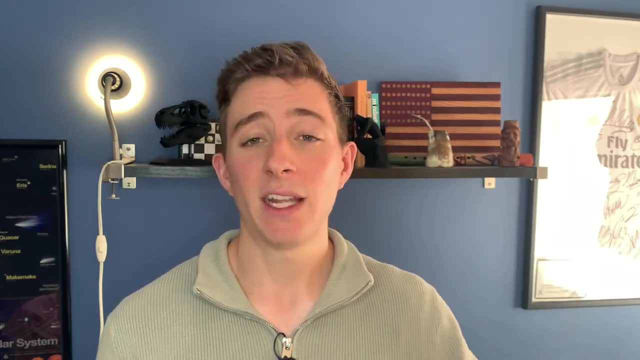 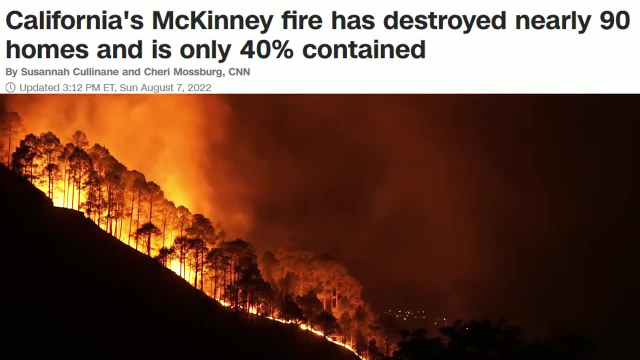 don't tend to hear a lot about in a place like California, Not to mention all the natural catastrophes that do tend to happen in California. You've got the wildfires, you've got the landslides, you've got the earthquakes, the volcanoes, the droughts and stuff like that. It's pretty brutal. 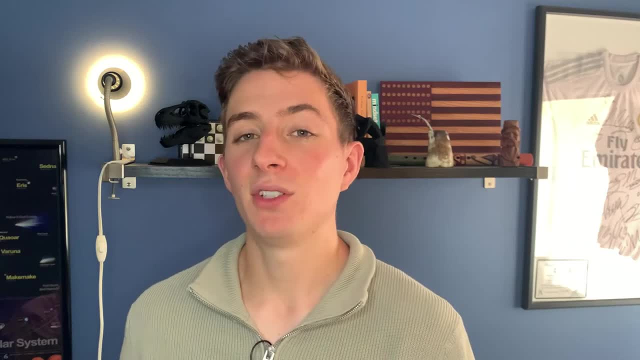 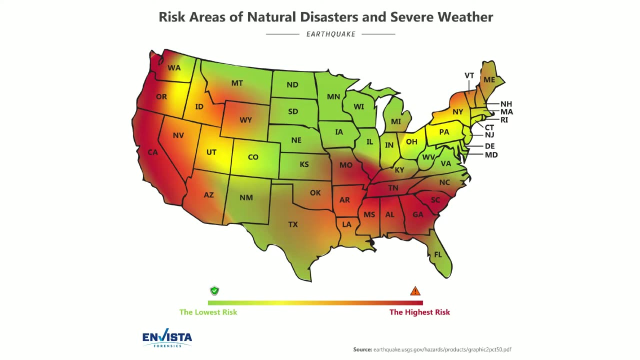 out there what can actually happen and what's been happening, Whereas here in Virginia, in Northern Virginia, you don't tend to experience any sort of natural catastrophes like California or even Tornado Alley in places like Texas- The worst thing I've experienced here-